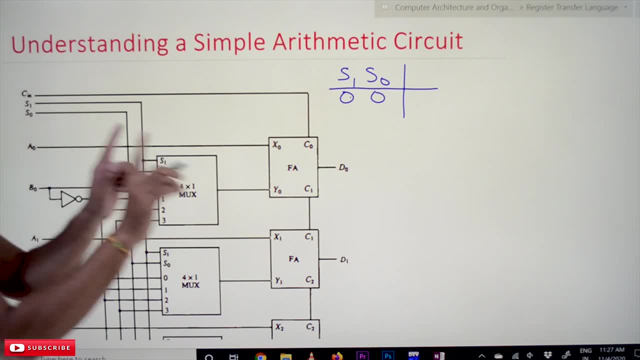 the input that is generated by the multiplexer. So whenever the value of S0 and S1 is 0, 0,, the 0th line of each and every multiplexer will get selected. So what is the input line that is connected to 0th input? The input that is connected to the 0th input is B value. 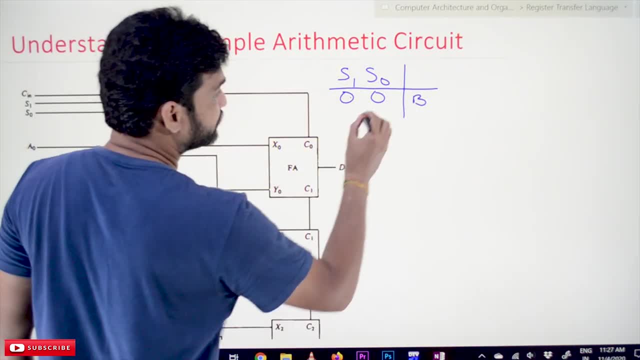 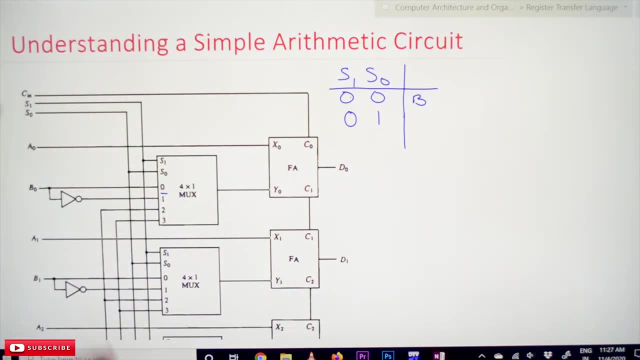 The value of B will be produced as the output Whenever the value of S0 and S1 is 1, 0.. So what is the output that it is going to produce? It is going to produce the complement of B. See here the 1 input line, the input line. 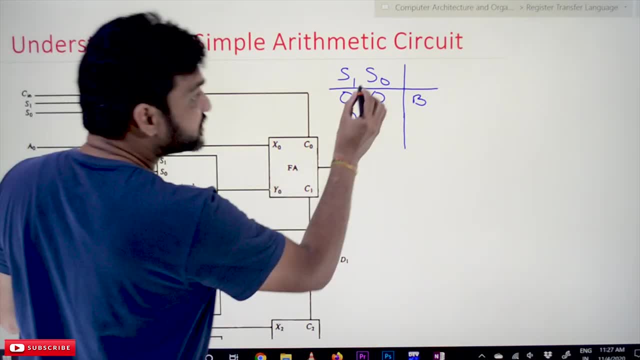 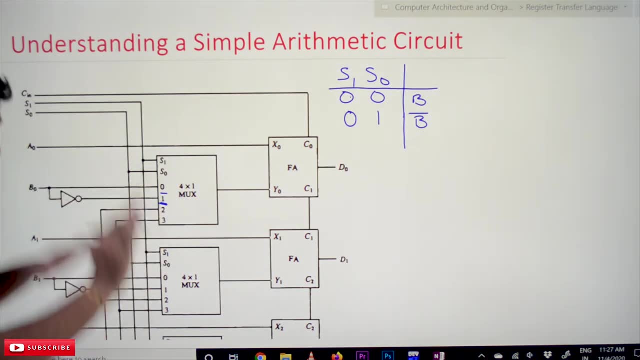 1 is connected with B complement. So whenever the value of S0 and S1 is 1, 0,, it is going to produce an output of B complement. Similarly, whenever the value of S0 and S1 is 0, 1,, what? 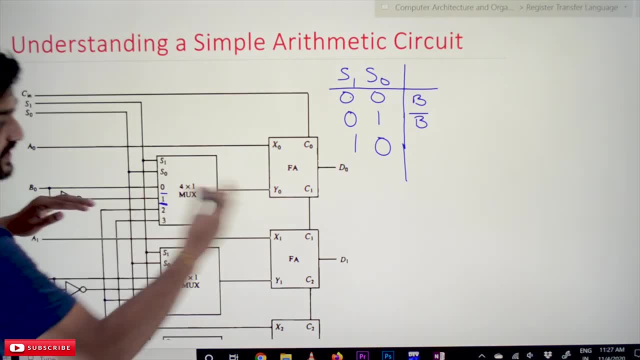 is the output that it is going to generate. The output generated by the multiplexer is. so what is the value that is generated by the multiplexer? Okay, The input line 2 is connected to the input line 2 is connected to 0.. See here. 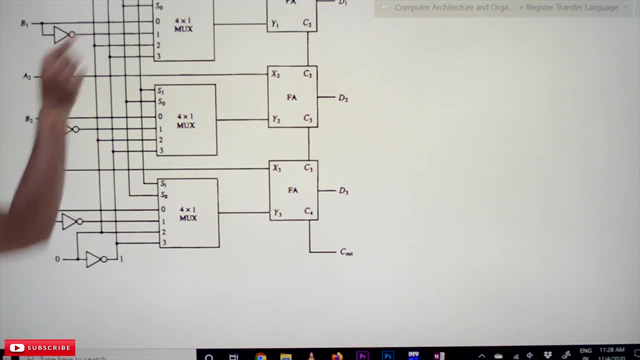 the input line 2 is connected to 0.. All the input lines 2s are connected to 0. And all the input lines 3s are connected to 1.. See, here, here we are having a circuit. It is continuously provided with 0 and it will get negated whenever the select line is, whenever. 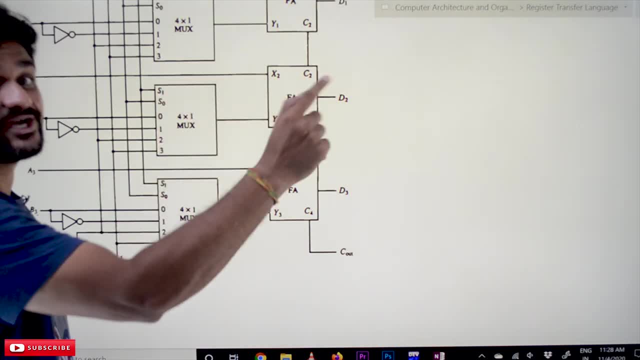 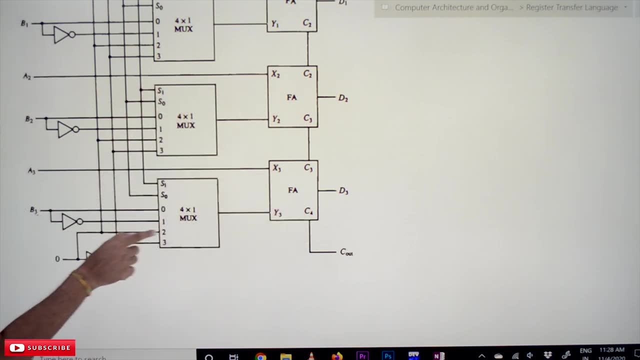 the select line S0 and S1 is provided with 0 and 1 is given. So each and every multiplexer of 1,, it is going to select the select line 2, which is provided with the input 0, see here 0 is provided and whenever the select line S0 and S1 is 1, 1, it is going to select. 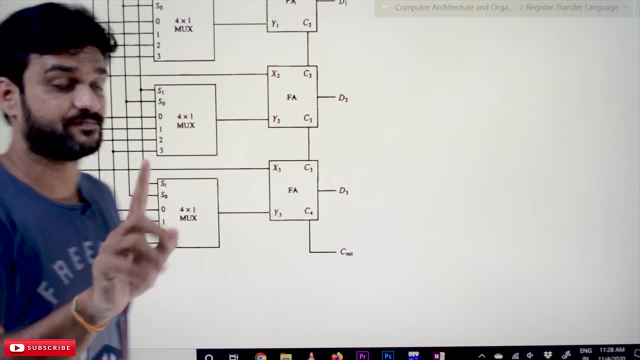 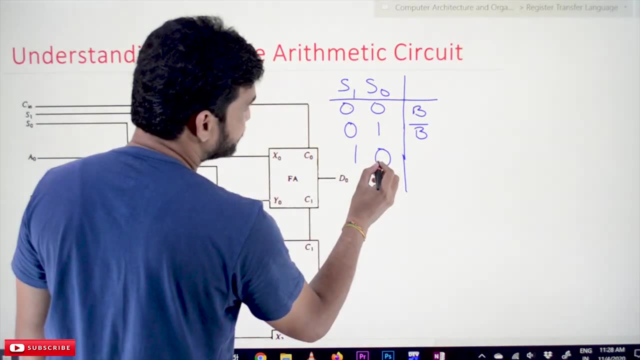 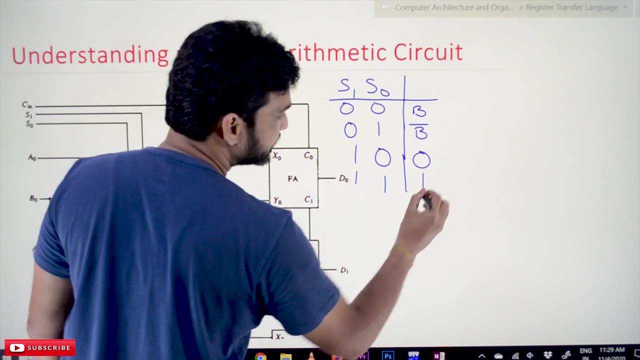 the select line 3, which is provided with an input of 1.. So now see here: whenever S0 and S1 is equal to 0- 1, it is going to select 0,. whenever the value of S0 and S1 is 1- 1, it is going to select the select line 3, which is provided. 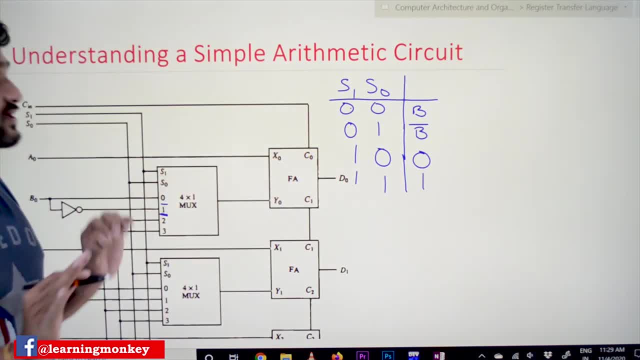 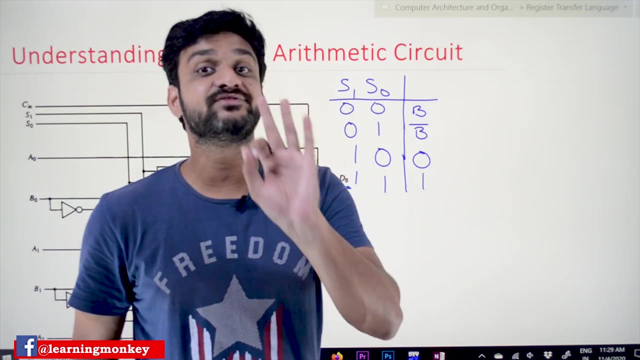 with an input of 1.. So now, what is how the value of D is generated by each and every full adder, how the value of how this value of D is generated by the full adder. a full adder is capable of adding. 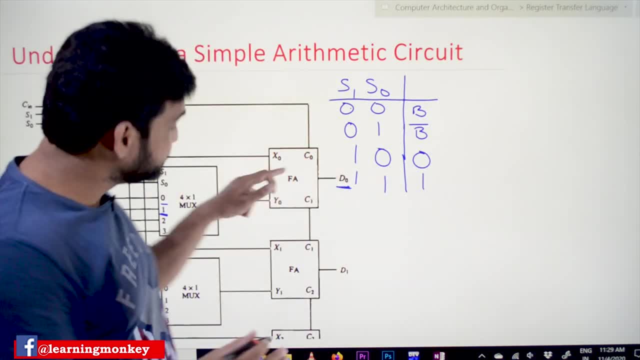 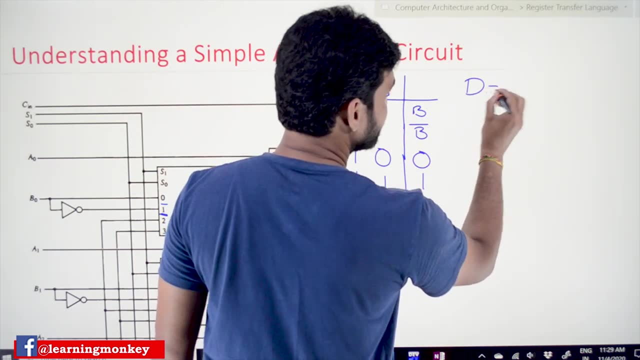 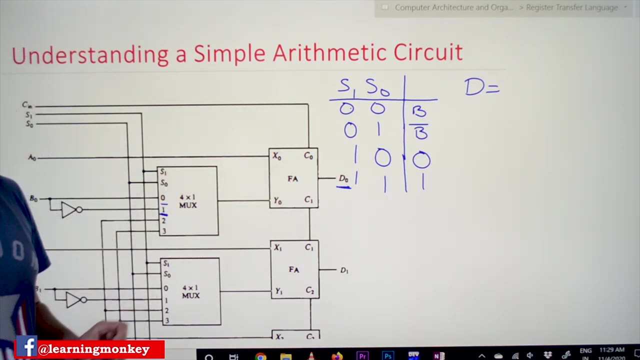 3 bits. What are the bits that are added by each and every full adder to generate the value of D? that we will try to understand and it is very important to understand. So the value of D on the full adder is generated by the sum of X0, Y0 and C0 in order to generate 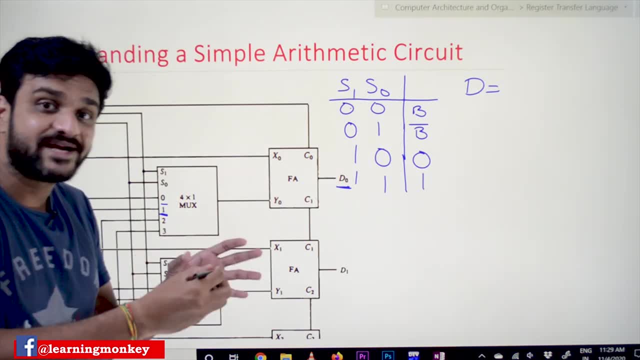 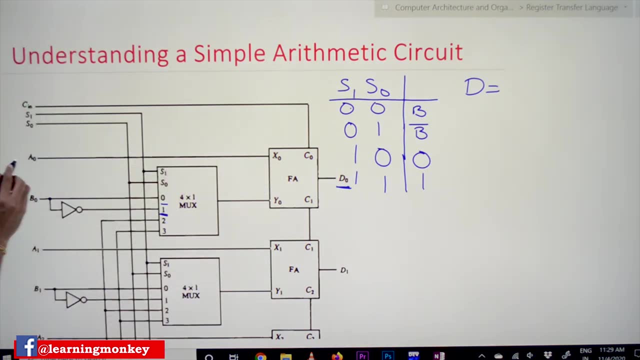 D0.. So what are the values that the that this full adder is going to add? it is going to add X0, Y0 and C0.. So the X0 value on each and every full adder is directly connected to A. 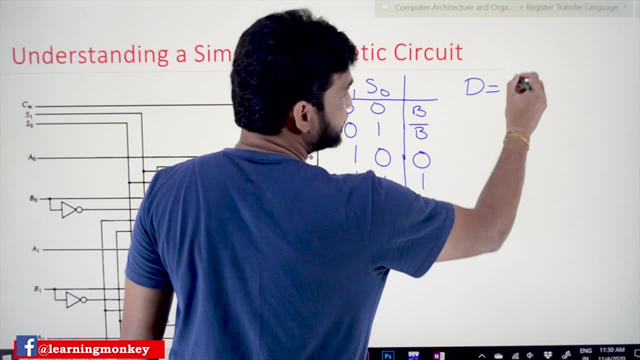 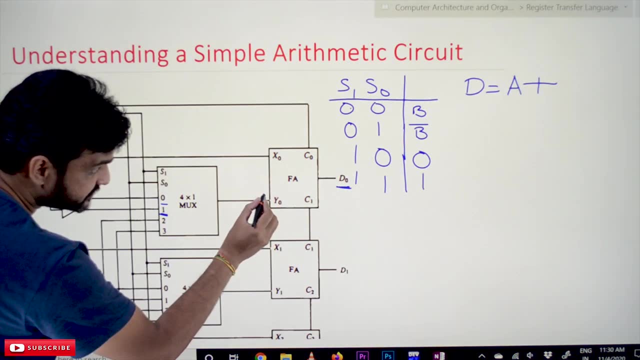 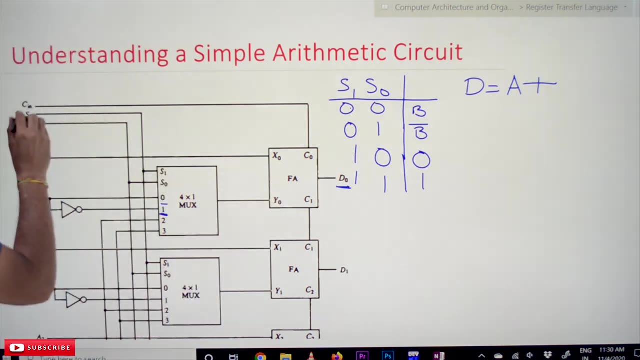 So, in order to generalize the terms, So the D is generated by adding the value of A plus it is going to. the D value is generated by the sum of A plus Y. How this value of Y is decided, It is decided by S0 and S1.. 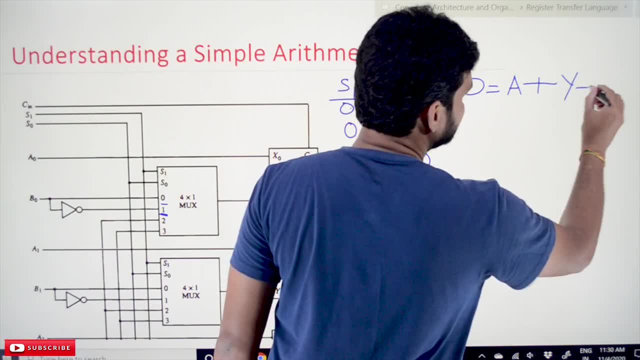 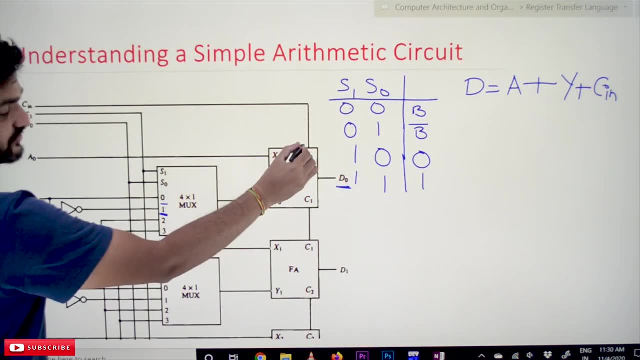 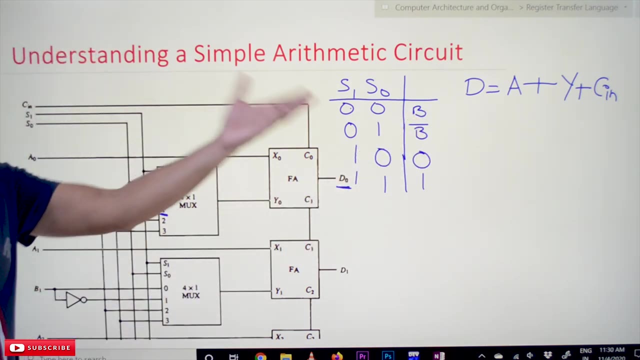 So the sum of A plus Y plus the next input is C in. What is the value of C in C in? the value which is provided by the C in C in C in is is one of the one of the value which decides the value of D. The value of D is: 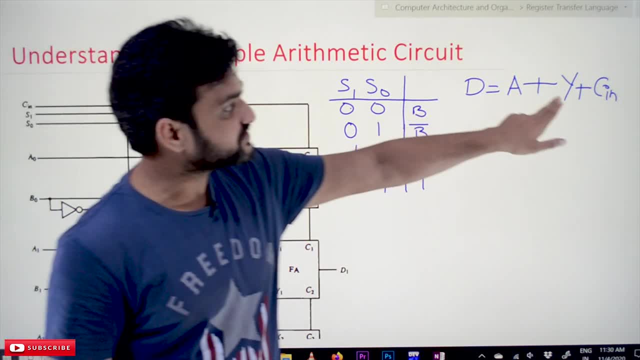 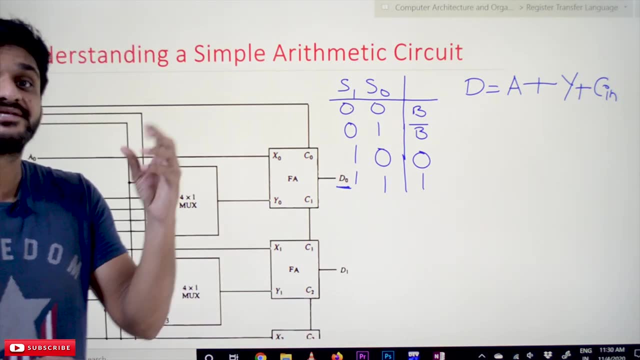 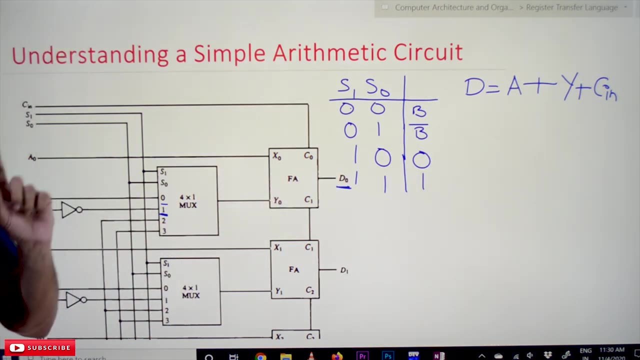 decided by X0, Y0 plus C0, which is A plus Y plus C in. So now, now, whenever the select lines and the C in is provided with the values, what are the operations that are performed by this circuit? That we will try to understand. 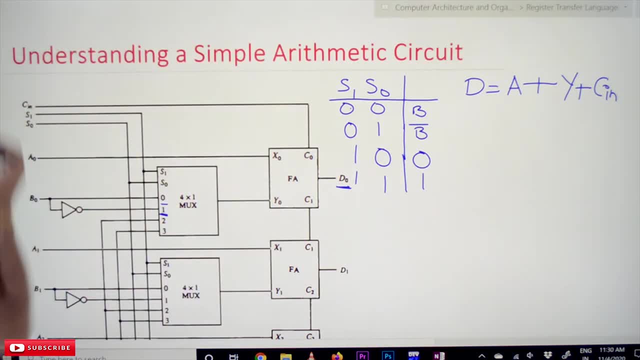 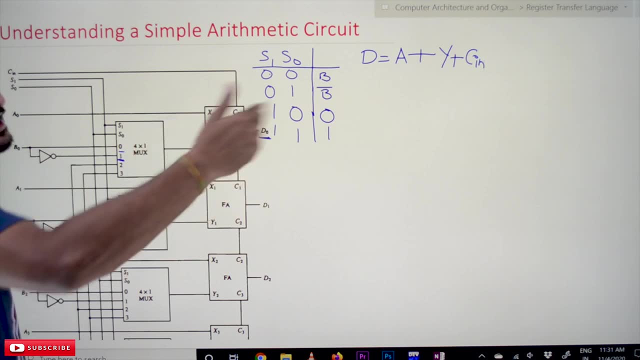 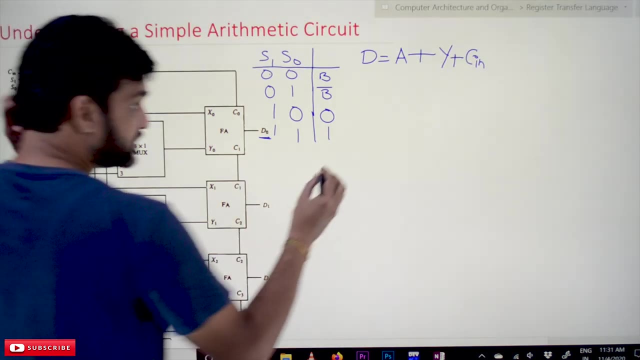 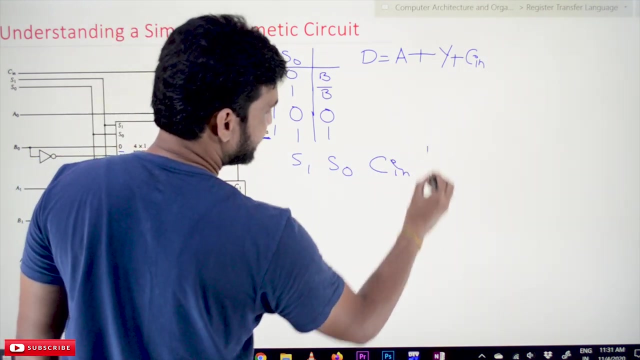 So how, what are the operations that are generated, That are performed by this circuit? That we will try to understand now, with the values of S0, S1 and C in. Saying it as C, it is C in. So whenever the value of S0, S1 and C in is provided with values. 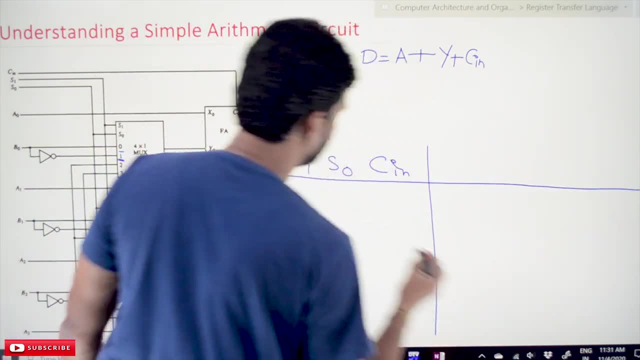 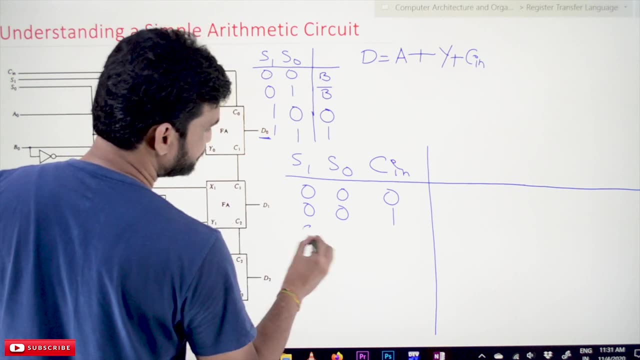 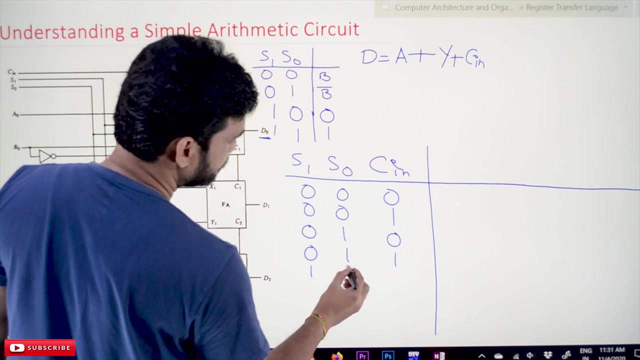 So what are the values that can be provided with S0, S1 and C in? It is 00.. So what are the values? It is 00.. 001.. The possibility, the possible values are 010,, 011, 100.. 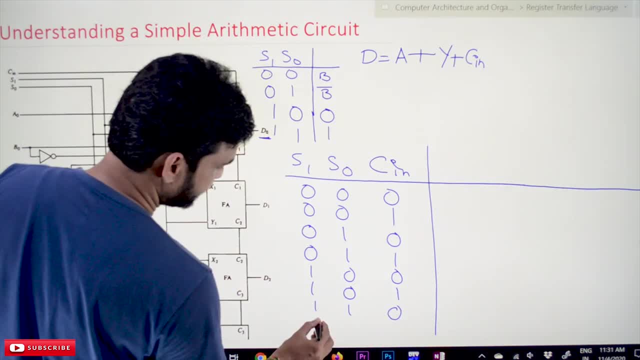 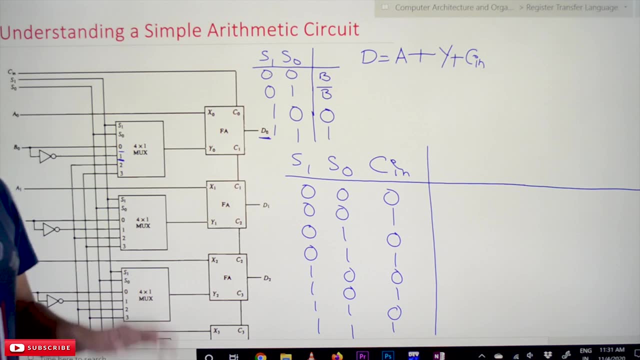 It is 101, 110.. And other possible value is 111.. So these are the values that can be provided to S0, S1 and C in. So whenever the value of S0, S1 and C in is 000.. 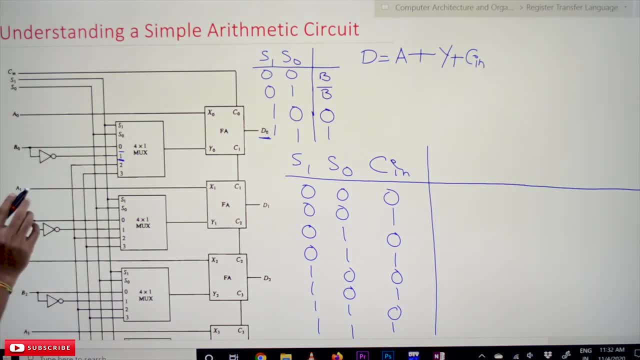 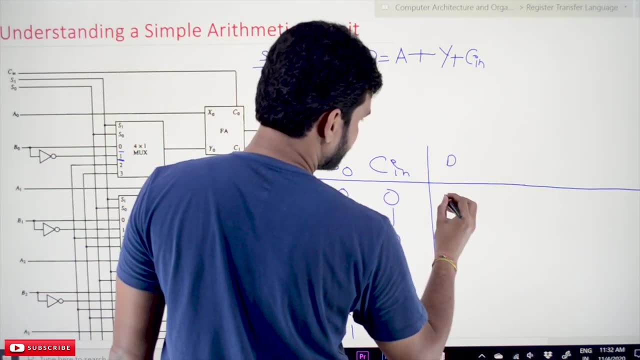 0, 0, 0.. So what happens? Whenever the value of S0 and S1 is 0, 0, the 0th input will get selected. So the value of D is equal to. the value of D is equal to A plus equation. 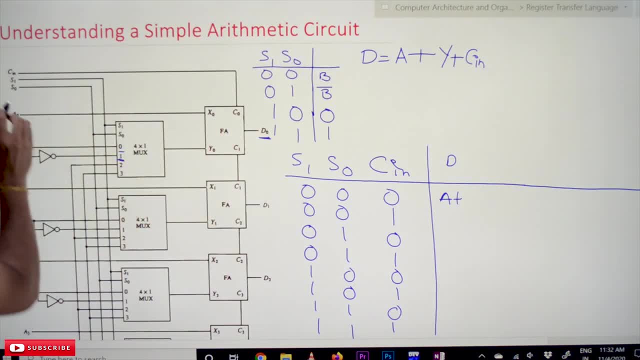 the value of it is going to be A plus. So whenever 0,, 0, 0 is provided for these values, what is the equation that is generated? It is A plus, So 0, 0 means the B input will get. 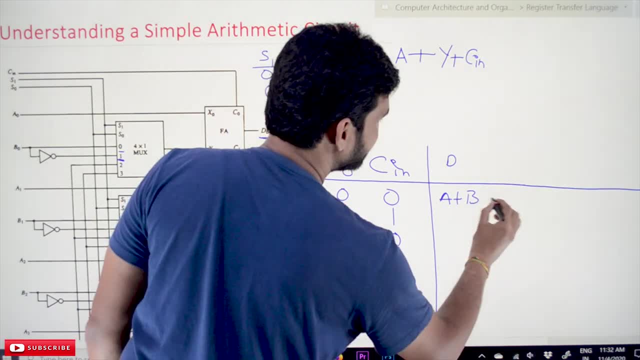 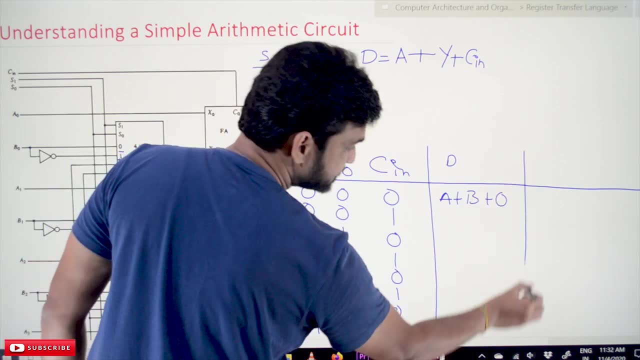 selected 0,. 0 means B input will get selected plus Cn is equal to Cin is equal to 0. So it is going to be A plus B plus 0.. A plus B plus 0 means whenever the value of S0, S1 and Cn is 0,. 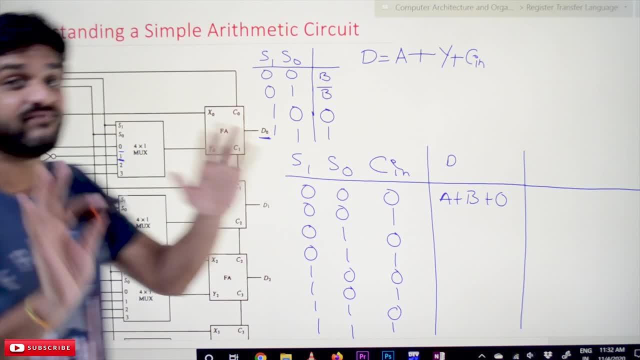 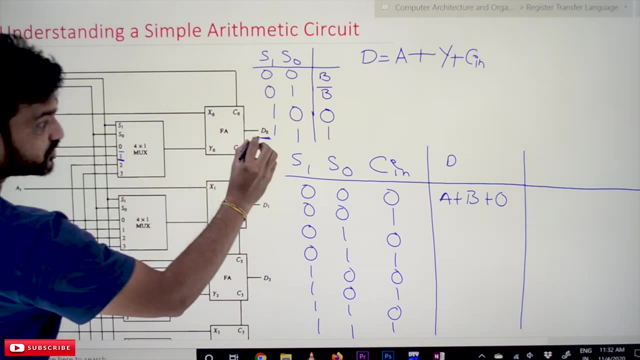 0,. it is going to add A plus B. The values of A and B will get added. See here: the value of A and B will get added and it is produced as the value of D. Okay, So what is? 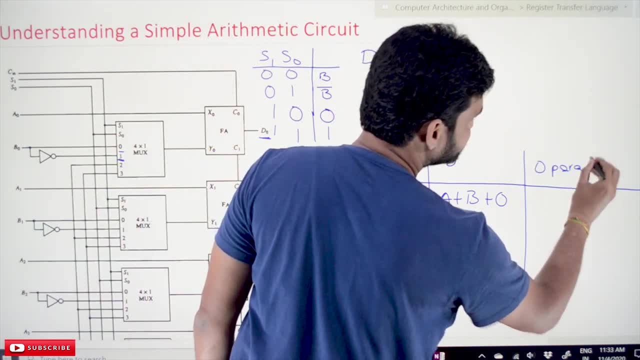 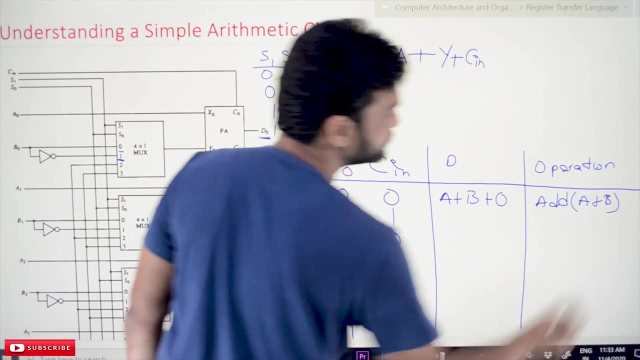 the operation that it is going to do. The operation is add, So it is going to add A plus B. So what is the operation? that is done Whenever the value of S0, S1 and Cn is 0, 0,. 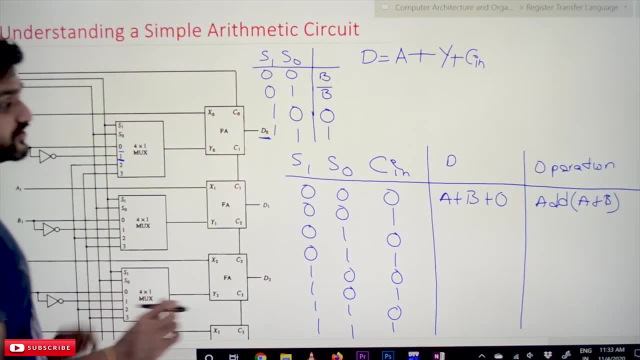 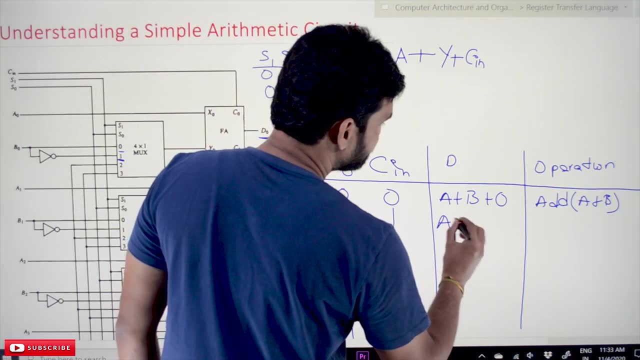 it is going to add A plus B. The next value is S0, S1 is equal to 0, 0 and Cn is equal to 1.. So it is going to be A plus B plus 1.. Okay. 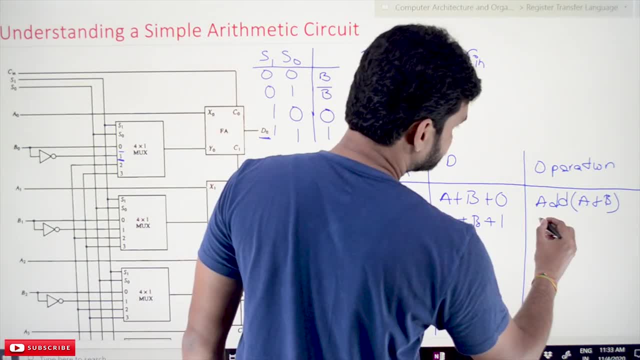 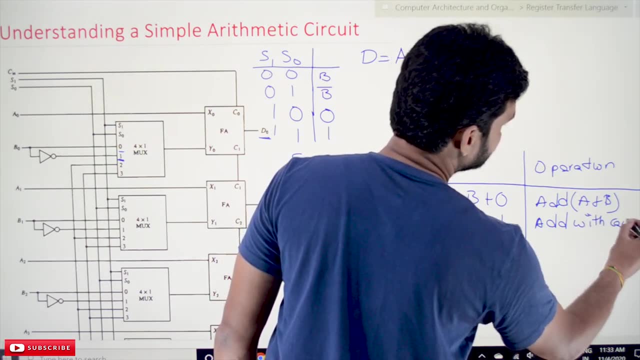 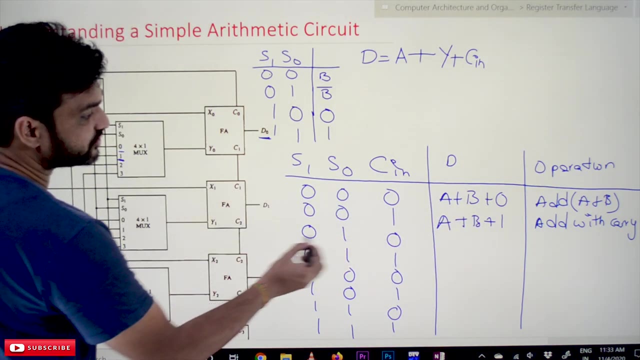 Okay, So it is add with carry. So it is going to add with a carry. The carry value is 1.. Whenever the S0, S1 is 0,, 1 and the Cn is 0. So what it is going to produce, So it is going to produce. 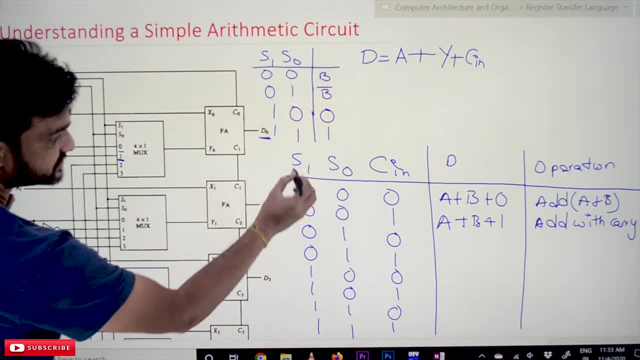 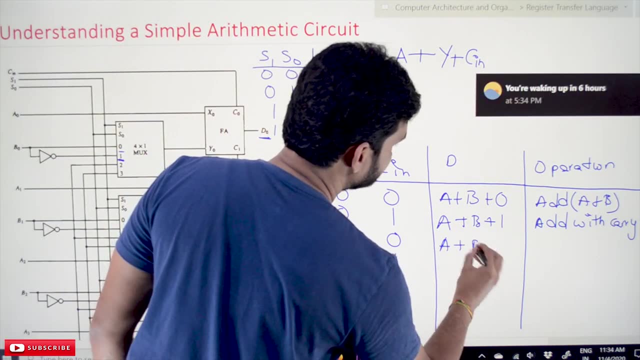 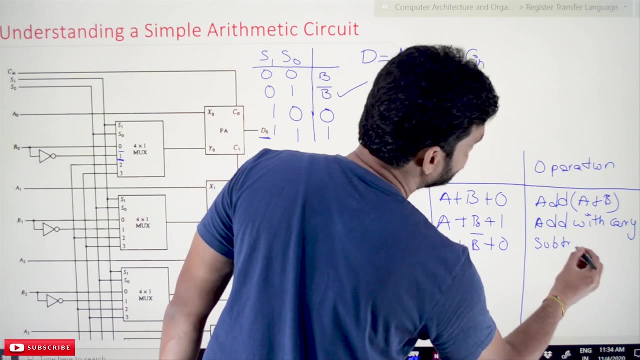 B complement. Whenever the value is S0 and S1 is 1, 0, 1, 0, it is going to produce B complement. So the equation is A plus B complement plus 0. So A plus B complement is subtract with a borrow. 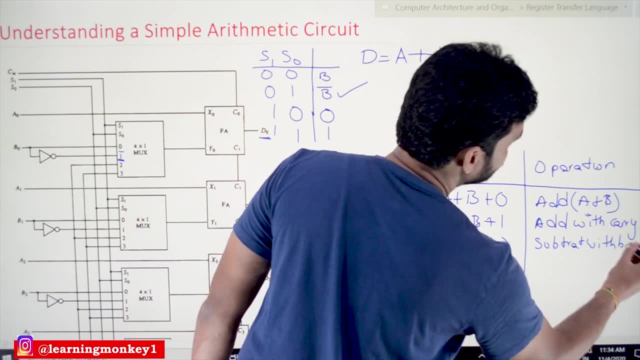 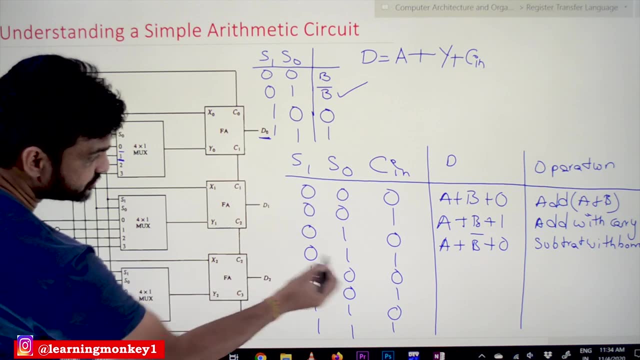 Subtract with borrow. The operation done is subtract with borrow, Whenever the value of S0, S1 is 0,, 1,, 0 and the Cn is 1.. So what it is going to produce, It is going to be A plus. 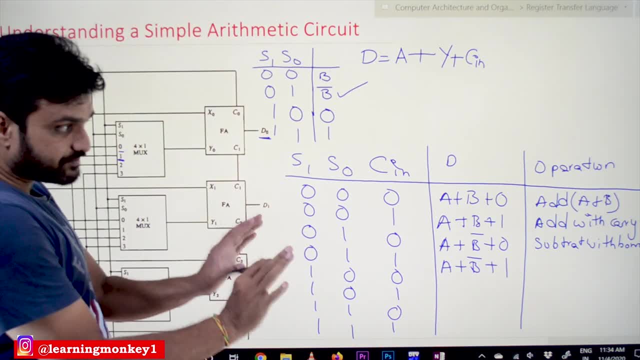 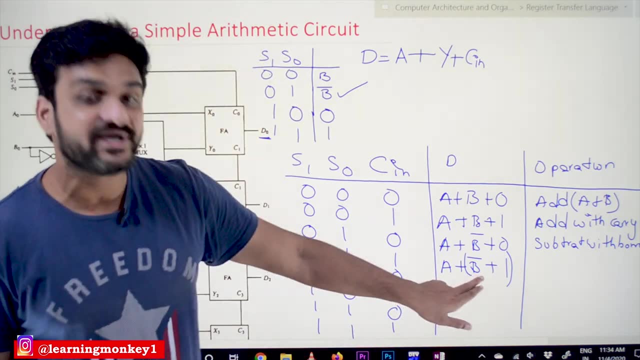 B complement plus 1.. So this is important point to understand. So B complement was plus 1.. So what this B complement plus 1?? It is the 2's complement of B. What is the 2's complement of B for a given value? If you find: 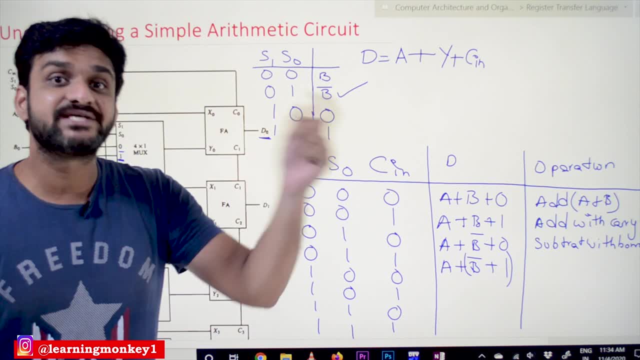 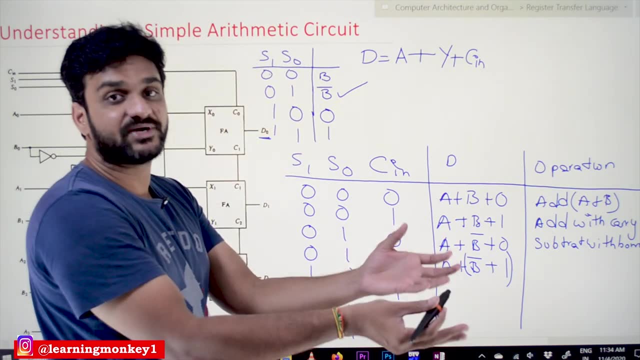 the 2's complement what it is going to be. It is B bar plus 1.. So B complement plus 1 is going to be the 2's complement. So adding A plus any 2's complement value is A minus B, See here. 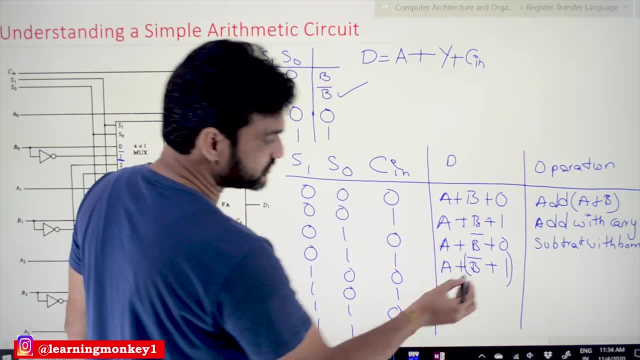 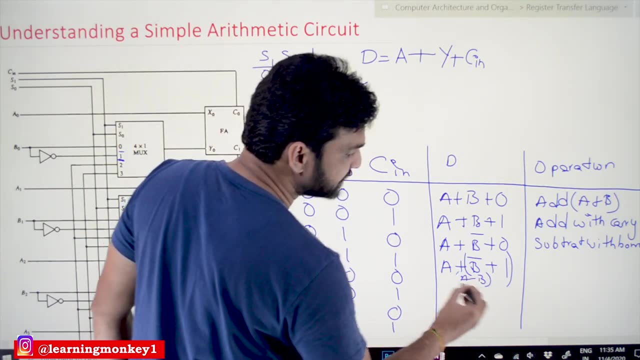 whenever we add A plus 2's complement of a value, it is going to produce B bar plus 1.. So any value plus 2's complement of another value, it is going to be A minus B. So this is going to subtract A and B. 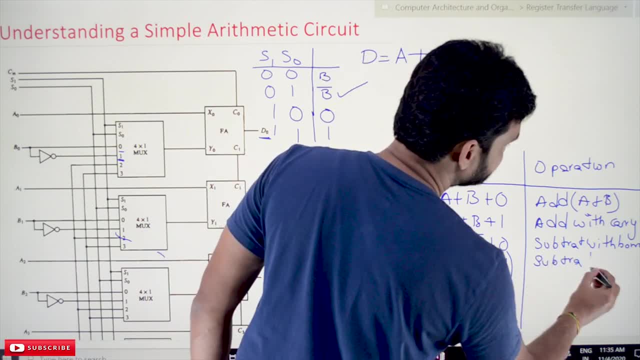 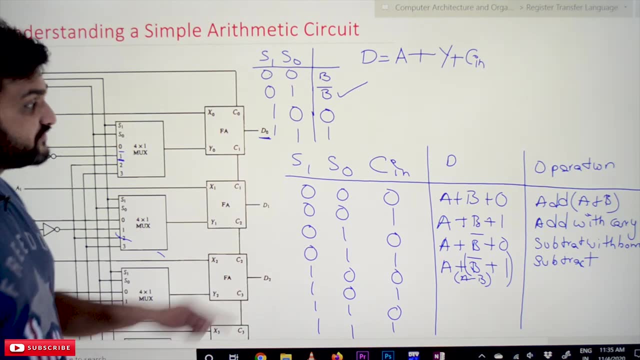 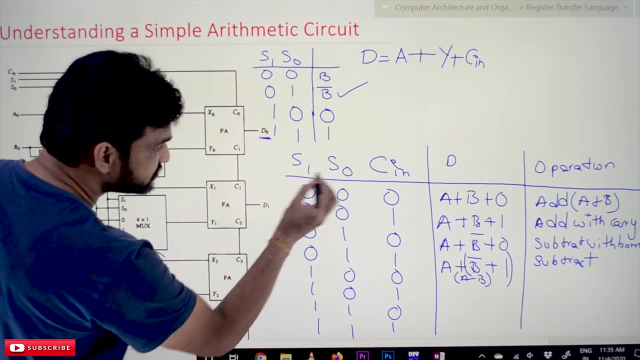 So the operation that is performed: it is going to subtract A minus B when the value of S0, S1 and Cn is 1, 0, 1.. Whenever the value of S0 and S1 is 0, 1, 0, what it is? 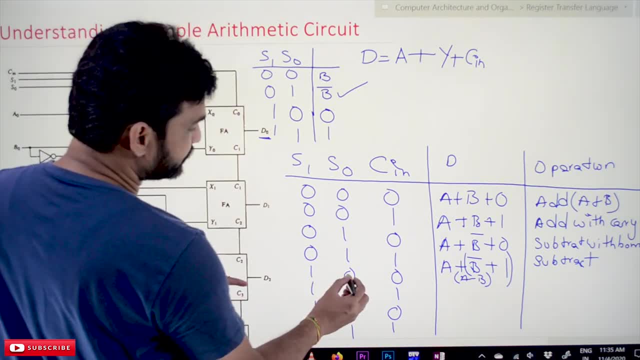 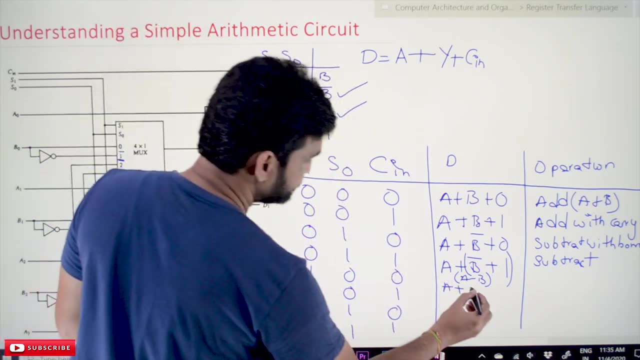 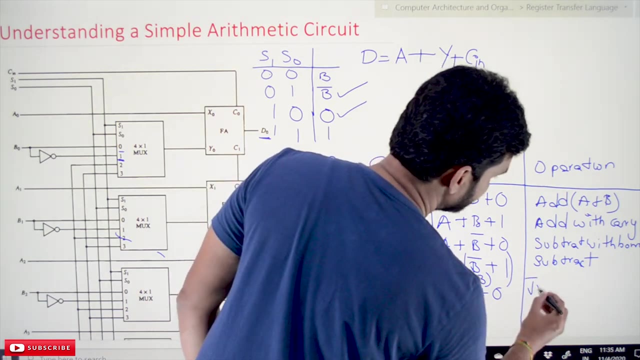 going to produce. So 0, 1, 0 means it is going to select 0. So it is going to be A plus the value of Y is equal to 0 plus 0. So it is going to transfer A. So what is the operation it is going to do? It is going. 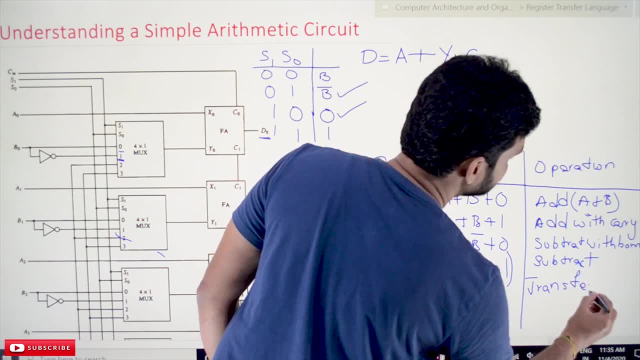 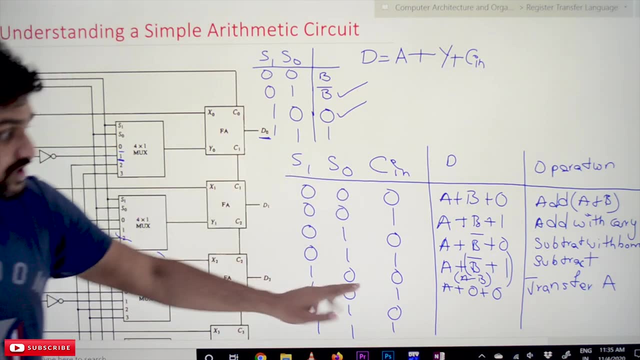 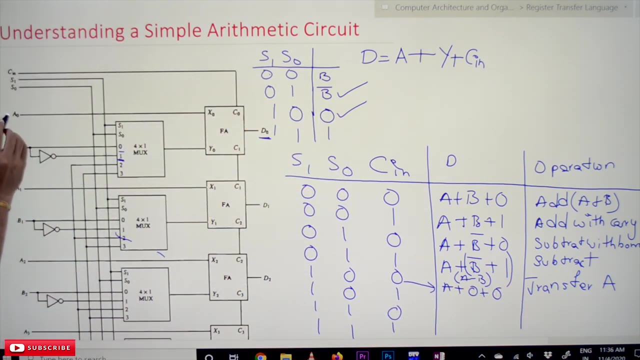 to transfer the value of A. Whenever the value of S0,, S1 is 0,, 1 and Cn is 0,, it is going to transfer A. The values that are present at A will be transferred as the output. If you want to transfer the value of A out of the circuit, just provide the values of. 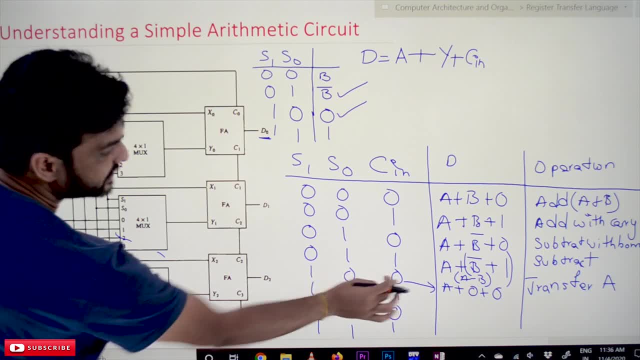 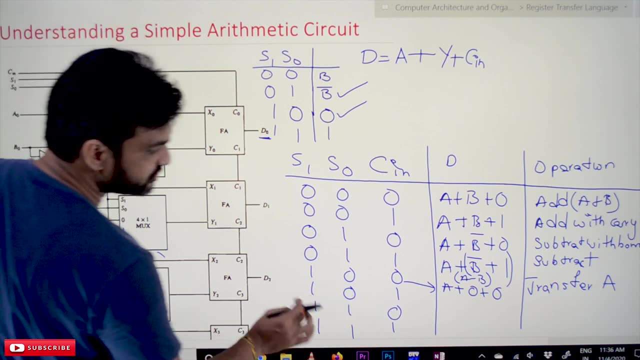 S0, S1 and Cn as 0,1 and 0. Whenever the inputs are 0,, 1 and 1,, the value of S0, S1 is 0, 1 and the CN is 1, it is A plus value of A minus S1 minus B. So it will drug like this: It will bend in and contract. So from here on you cannot such roast and set step for A: 1,, 2, 3, 4, 5, 4, 5,, 6,, 7, and 10,. no second over B B is taken. G A is the, that is 40 degrees. 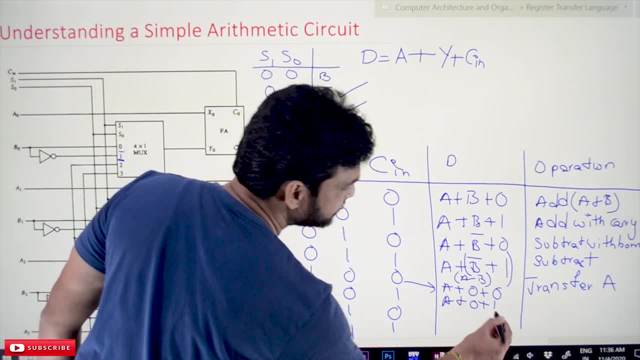 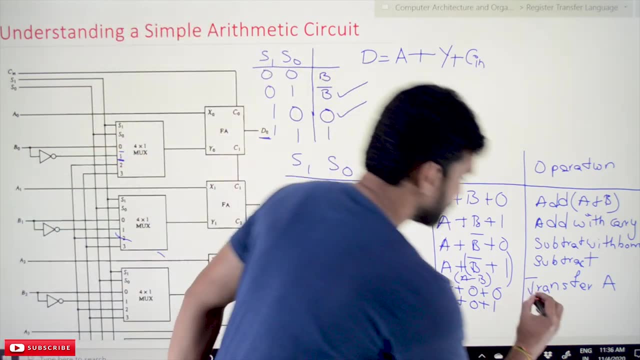 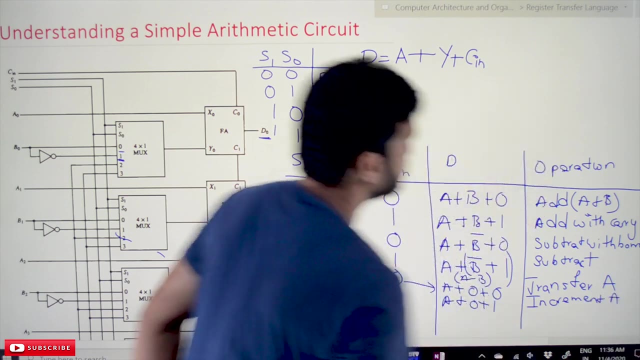 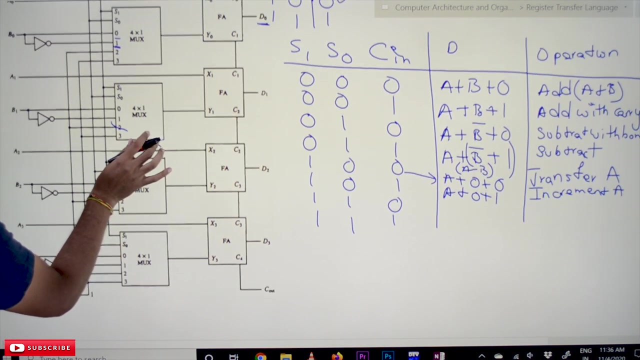 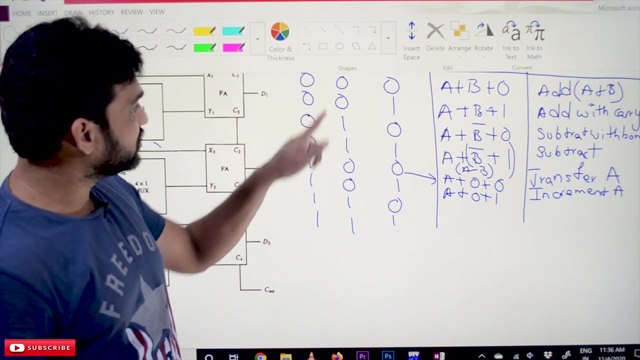 the value of y is 0 plus 1.. So what it states is: increment the value of 1, increment the value of a. It is going to increment a, So let us expand this. increment the value of a in And whenever the value of s0 and s1 is 1, 1, s0 and s1 is 1, 1 and c in is 1.. So 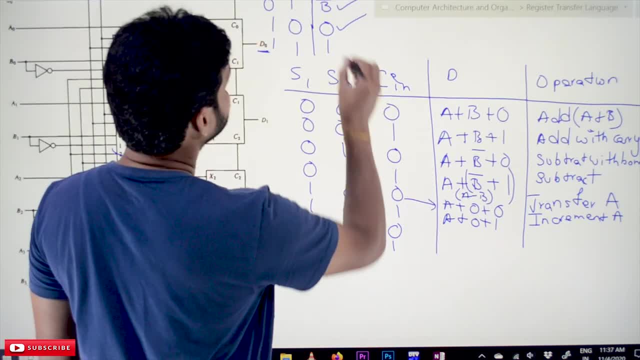 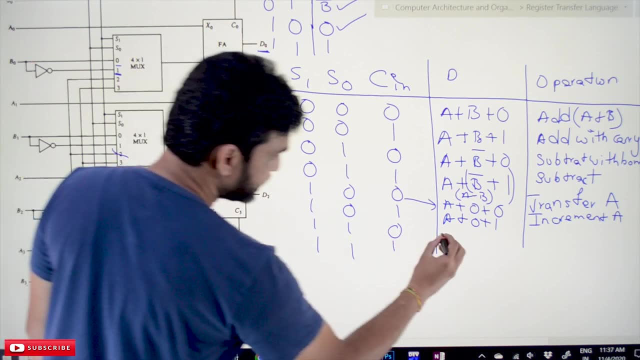 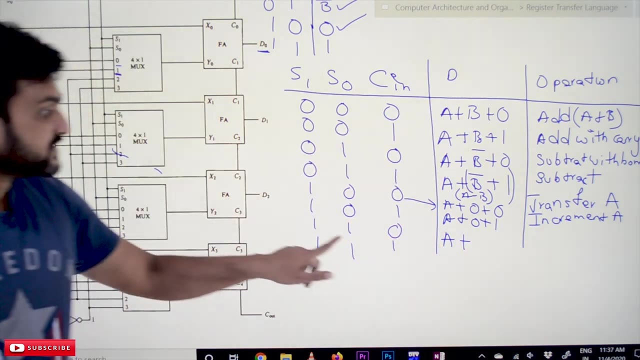 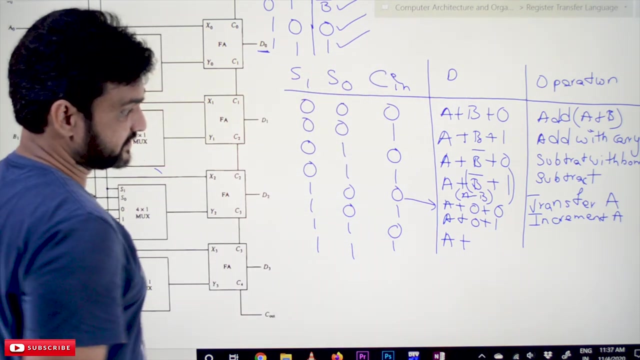 what it is going to produce as the output. So what it is going to produce as the output- It is a- is common for all the values plus the value of y. The value of y is decided by the value of y. So the value of s0 and s1 is 1, 1.. So it is going to be 1. a plus 1 plus 0. See here. 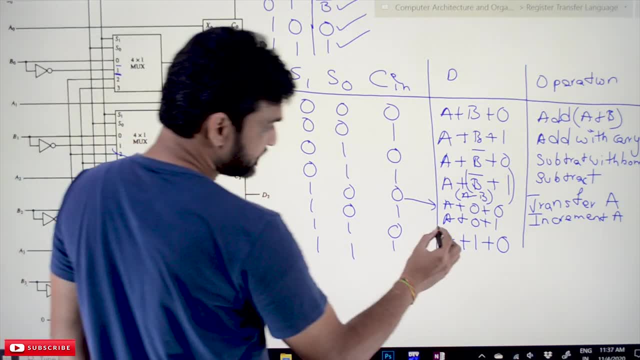 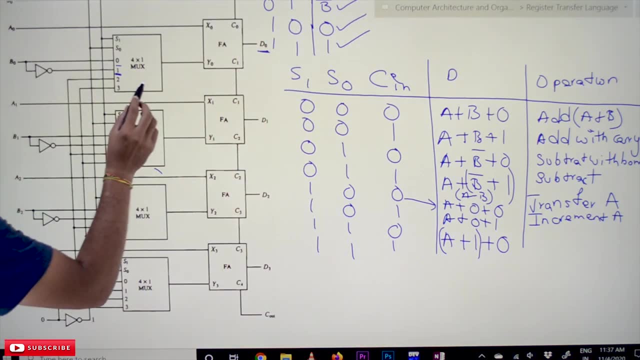 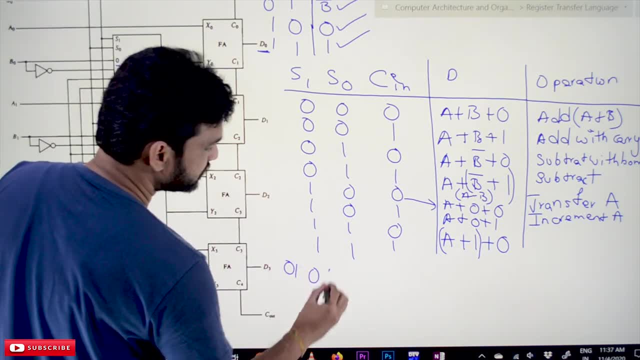 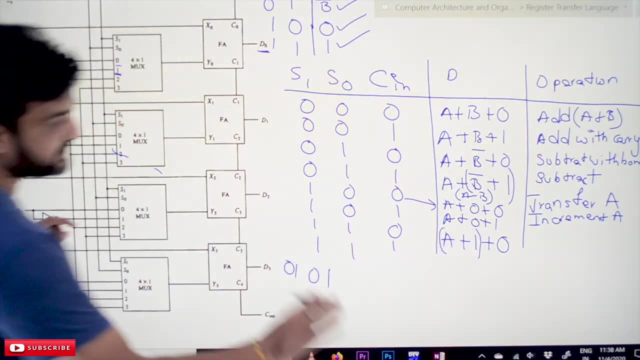 and here the value of a is 1, 0, 1, 0, 1, 0, 1.. If this is the value of a, a plus 1.. So here what this a plus 1 means is. a plus 1 means is so for every value of a, for every. 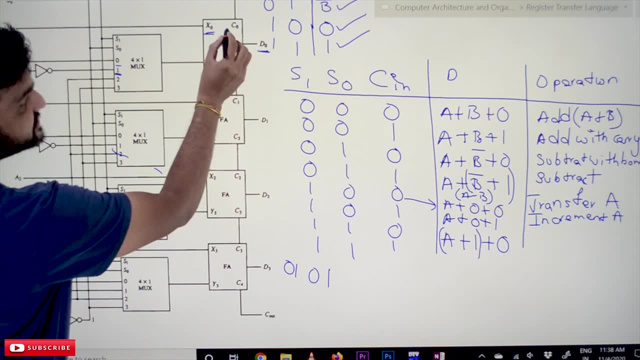 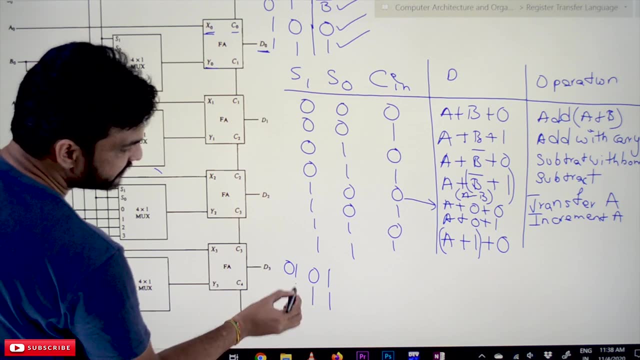 value of a, 1 is added and the c in is 0. So a plus 1.. So for this bit, 1 is added. For this bit, 1 is added. For this bit, 1 is added. And for this bit also, 1 is added. 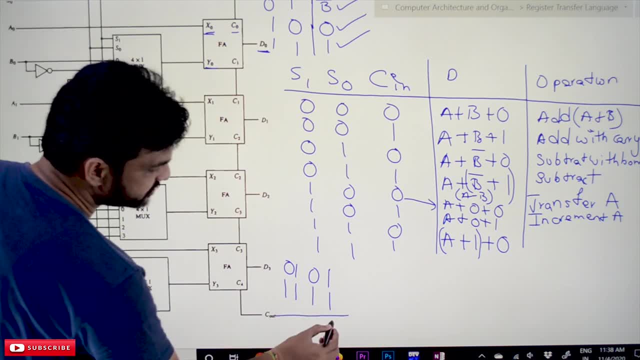 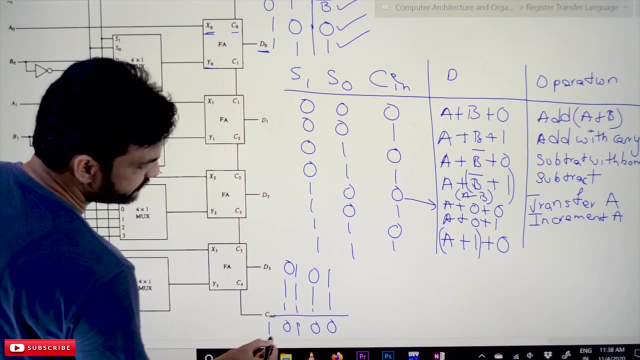 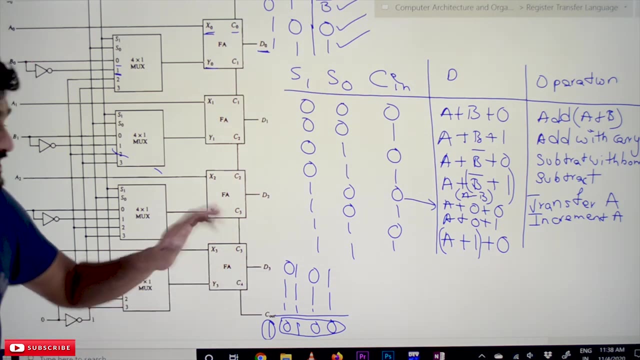 is added. So let us see the output of this. It is going to be 0, 1.. It is 0, 1, 1, 1, 0, 1.. So this is carry out. So the value is 0, 1, 0, 1, 0, 0.. So what is happening here is whenever. 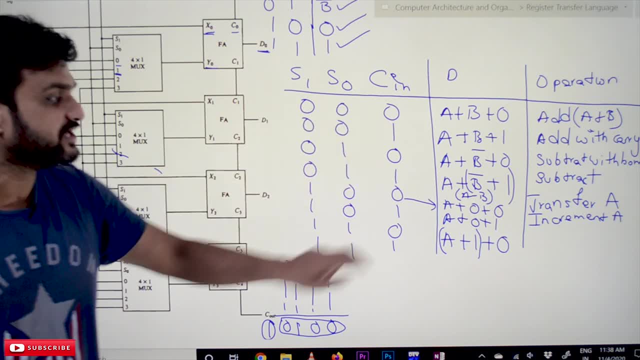 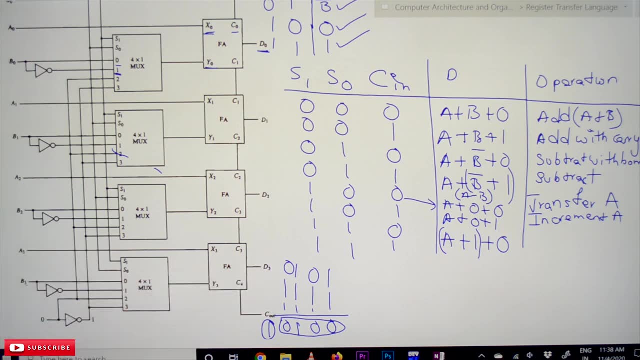 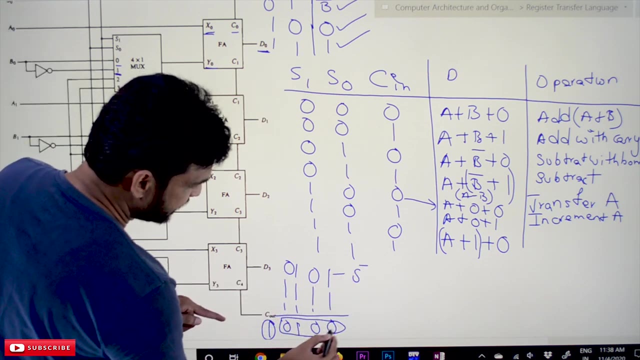 the inputs of S0, S1 is 1, 1 and the CN value is 0,. what is happening is it is going to do, it is going to perform decrement of here. So here the value is 5 and the output that we are going to get is 4.. So how we are going to decrement is: So what is this? This is. 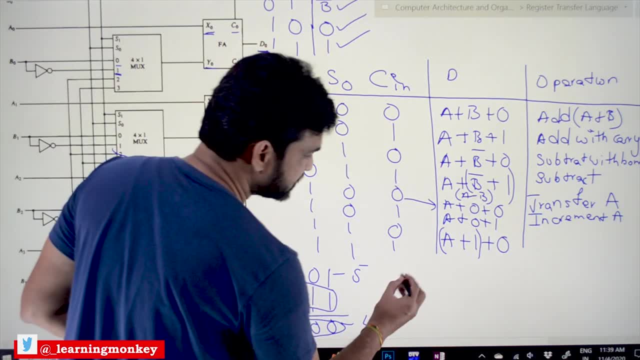 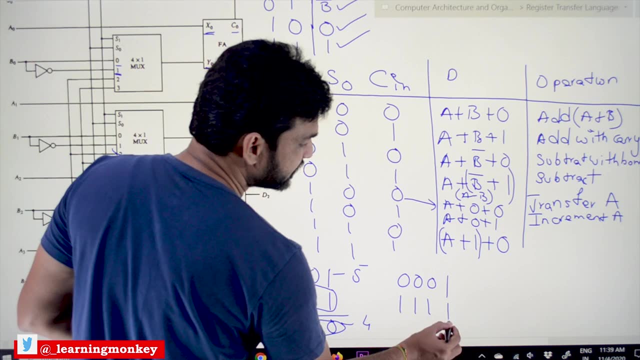 the 2s complement value of 1.. So if you take 4 bit 0, 0, 1, what is the 2s complement of it? The 2s complement of it is going to be 1, 1.. Whenever we add: whenever we add. 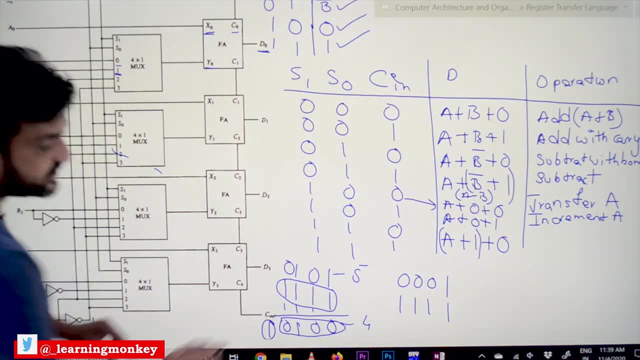 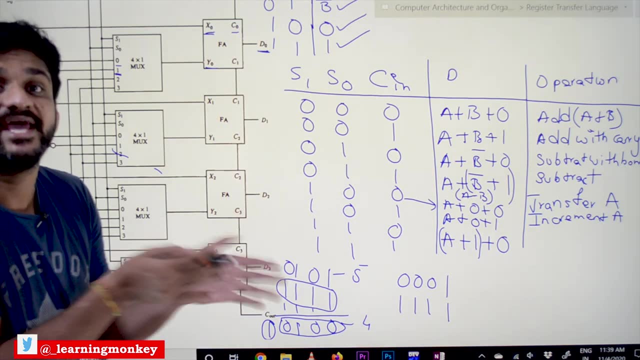 we add 1, 1, 1 to it. so 1 1 to it means a minus 1 is a minus 2's complement of 1 is added means it is a minus 1. okay, so the this value. so this is very important to understand. watch this again. 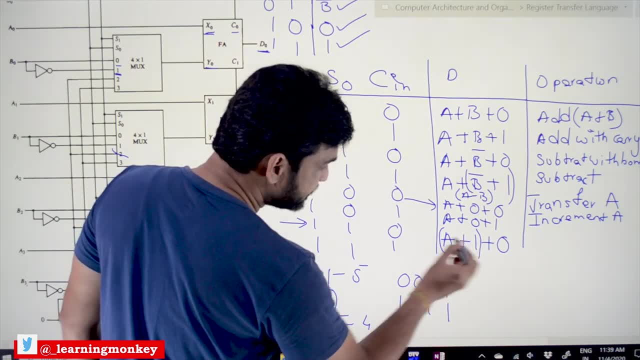 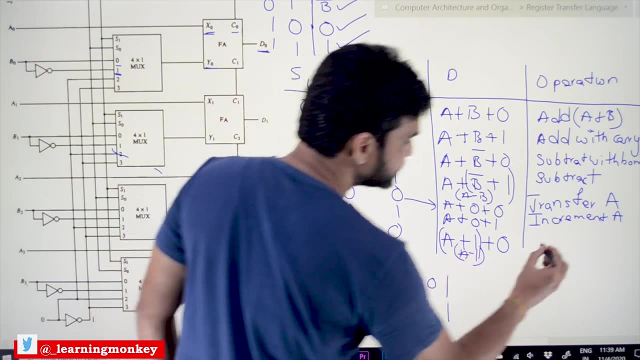 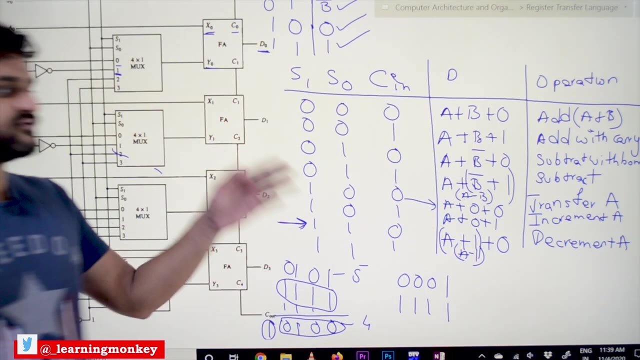 and again. so it is a, a, a, my, the, the. the operation that is performed by this is: it is a minus 1, which is a decrement a. we are going to decrement the value of a by 1. so whenever s naught and s, 1 is.